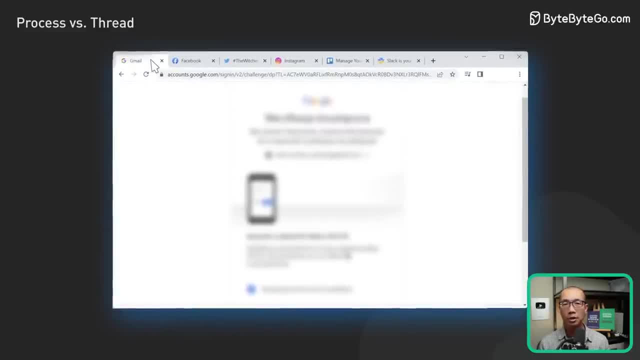 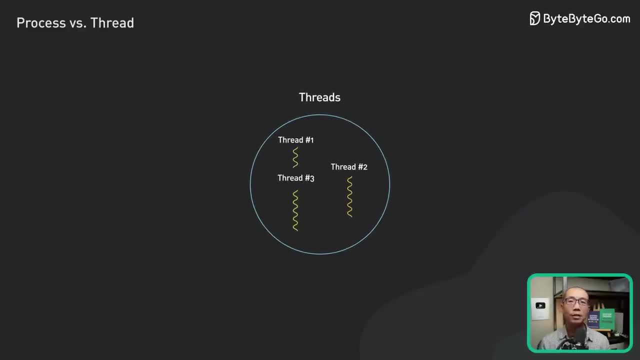 When one tab misbehaves due to a bug or a malicious attack, other tabs are unaffected. What is a thread? A thread is the unit of execution within a process. A process has at least one thread. It is called the main thread. 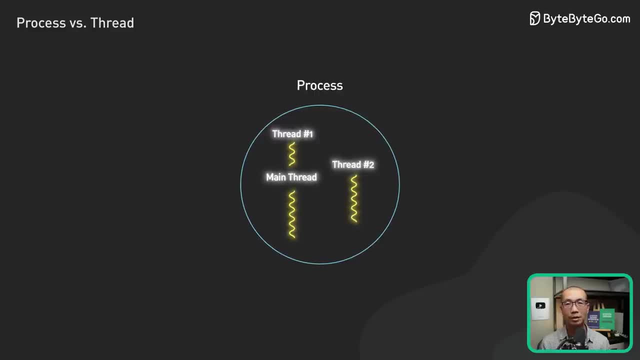 It is not uncommon for a process to have many threads. Each thread has its own stack. Earlier we mentioned registers, program counters and stack pointers as being part of a process. It is more accurate to say that those things belong to a thread. 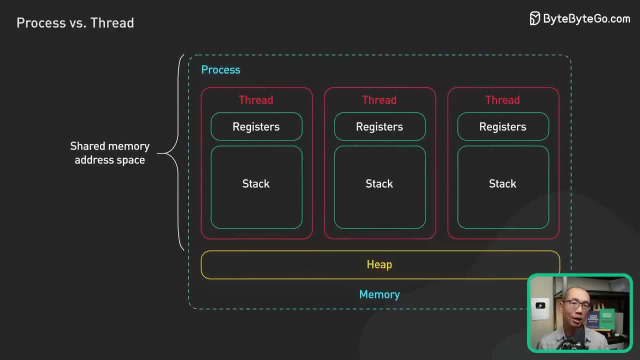 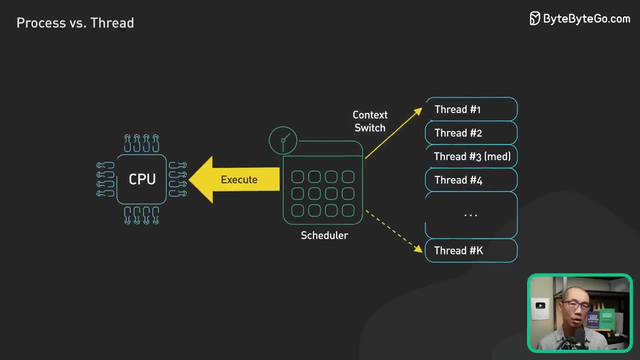 Threads within a process share a memory address space. It is possible to communicate between threads using that shared memory space. However, one misbehaving thread could bring down the entire process. How does the operating system run a thread or process on a CPU? 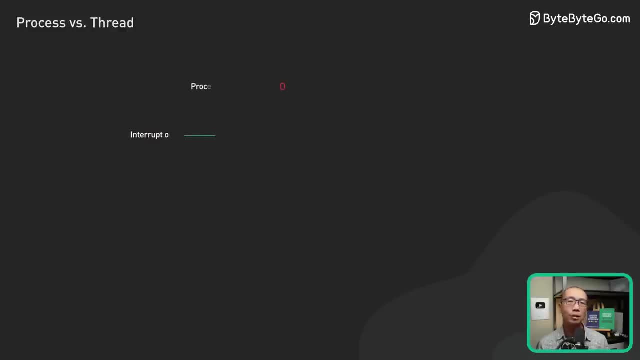 This is handled by context switching. During a context switch, one process is switched out of the CPU so another process can run. The operating system stores the states of the current running process, so the process can be restored and then resume execution at a later point. 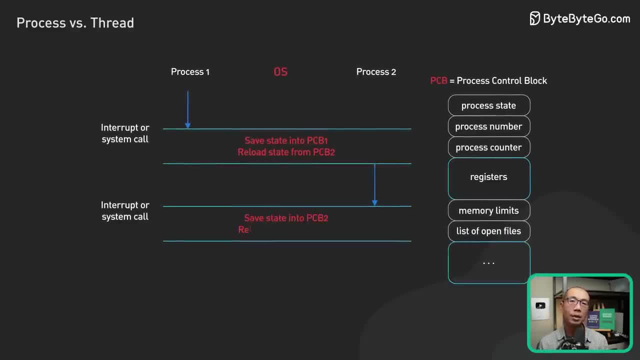 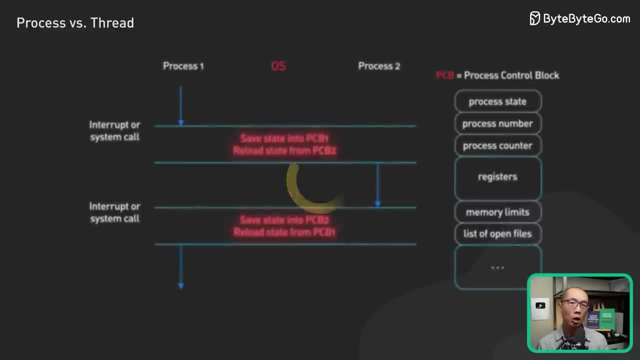 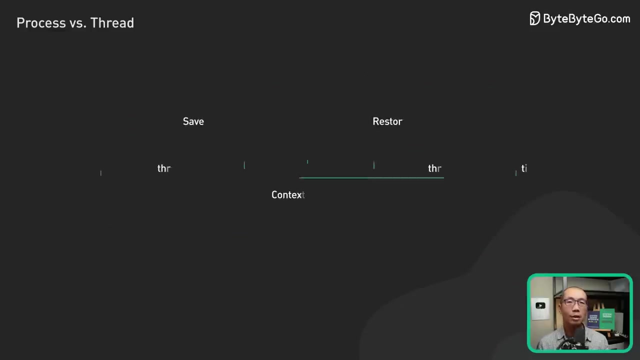 It then restores the previously saved states of a different process and resumes execution for that process. Context switching is expensive. It involves saving and loading of registers, switching out memory pages and updating various kernel data structures. Switching execution between threads also requires context switching. 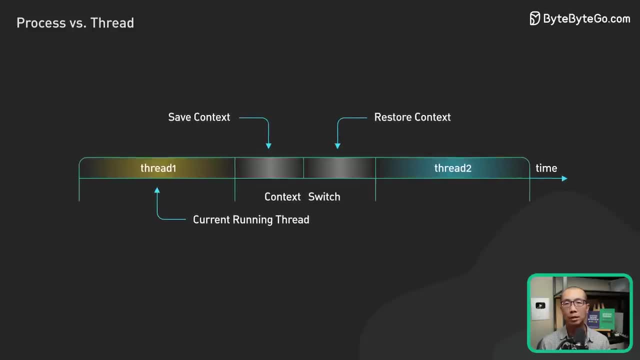 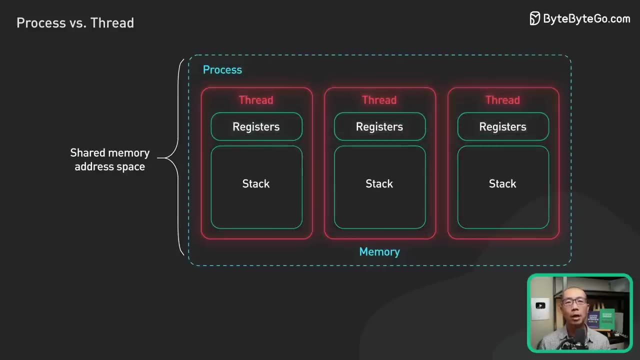 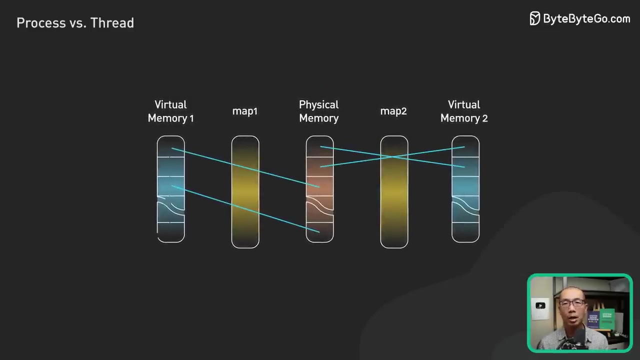 It is generally faster to switch context between threads than between processes. Therefore, there are fewer states to track and, more importantly, since threads share the same memory address space, there is no need to switch out virtual memory pages, which is one of the more expensive operations during a context switch. 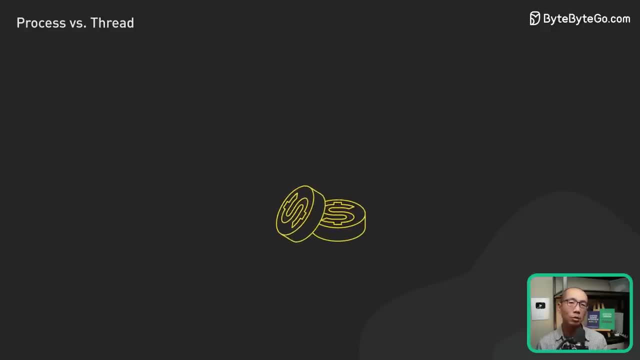 Context switching is so costly, there are other mechanisms to try to minimize it. some examples are fibers and coroutines. These mechanisms trace complexity for even lower context switching costs. In general, they are cooperatively scheduled, that is, they must yield control for others to run. 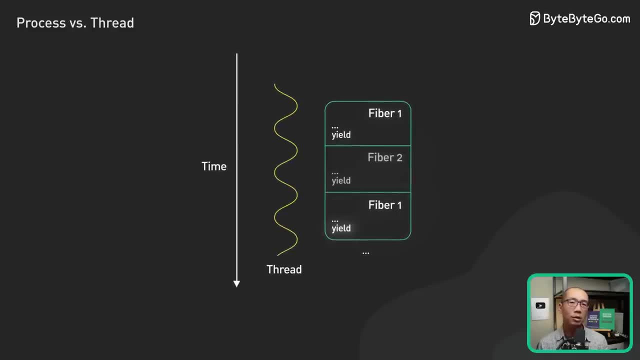 In other words, the application itself handles task scheduling. It is the responsibility of the application to make sure a long-running task is broken up by yielding periodically. This concludes our discussion of process and threads. If you'd like to learn more about system design,